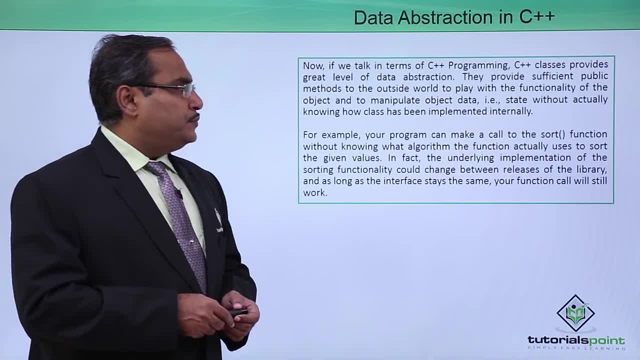 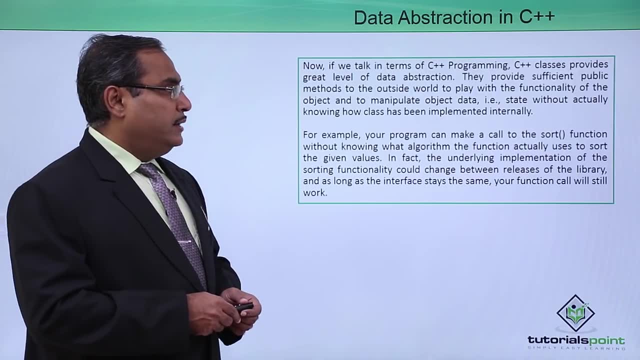 obstruction. But if we talk in terms of C++ programming, C++ classes provide a great level of data abstraction. They provide sufficient public methods to the outside world. So C++ will be the only one. So in this particular case, if we talk about the Internet, what we do? 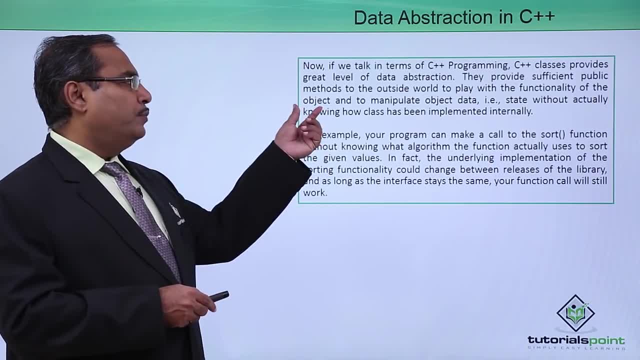 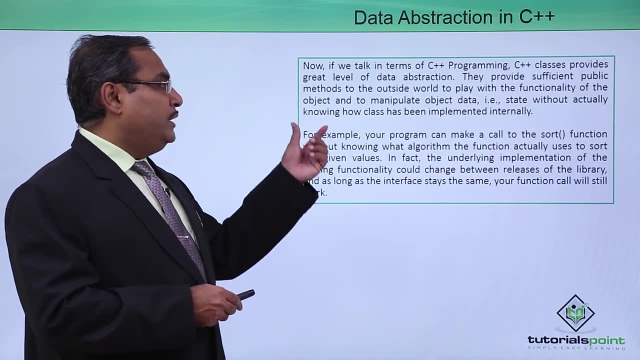 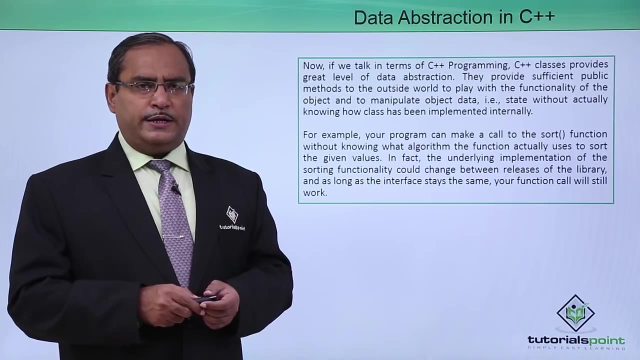 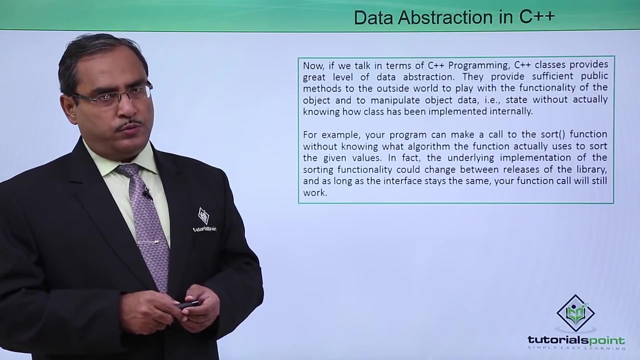 world to play with the functionality of the object and to manipulate object data, that is, state, without actually knowing how class has been implemented internally. so different methods will be retained in a certain object and those methods will be accessible, will be made accessible to the outside world. so when those methods will be accessed, how those methods are internally coded. 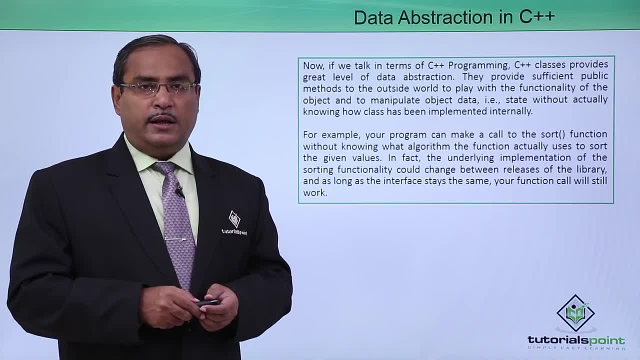 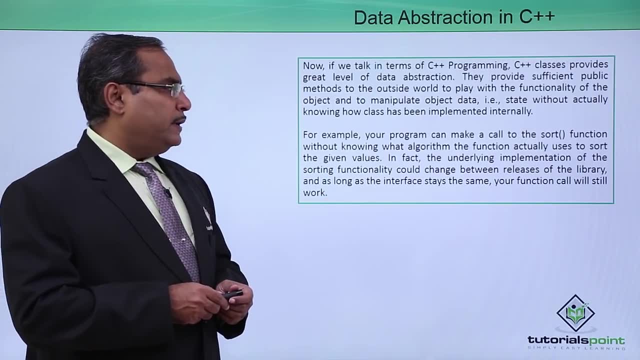 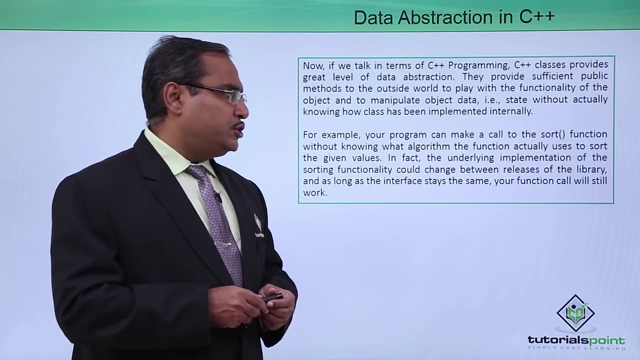 how those methods have got internally implemented. that will remain hidden to the respective user of the object. for example, your program can make a call to the short function without knowing that what algorithm the function shot is actually using and how the given data is getting shorted. in fact, the underlying implementation of the shorting functionality would change between 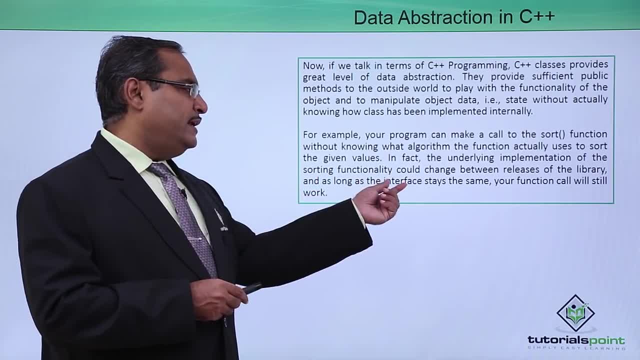 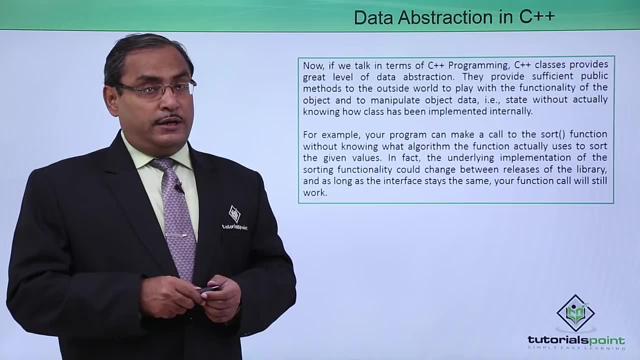 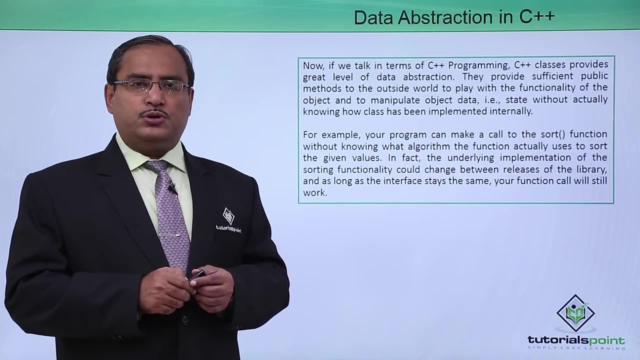 releases of the library and as long as the interface stays the same, your function call will still work without having any difficulty. in case of short function, we have taken this short function as an example. the internal code of the short function is totally unaccessible from the outside world. what shorting algorithm we have used? how the logic has been? 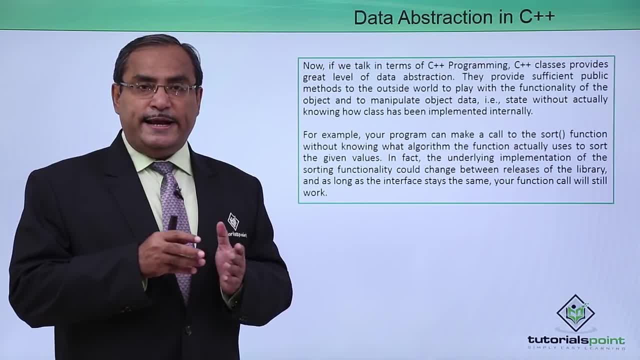 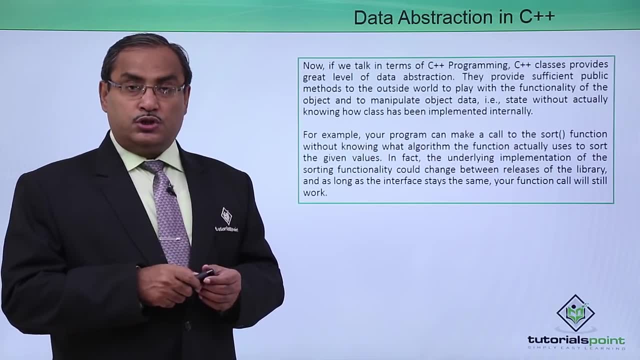 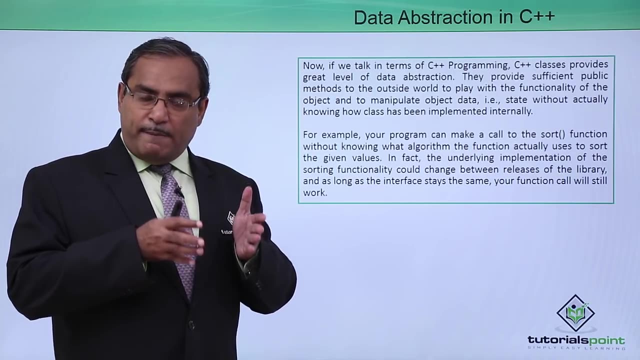 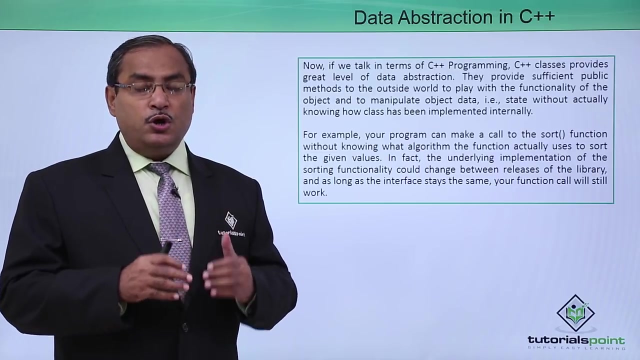 coded and how the data are getting shorted in intermediate scans so that those details will remain hidden to the outside world. so with the change in the release and version of the library functions, so this short algorithm, which was implemented internally, may have got changed, but if the interfacing remains the same, then the user who is calling the short function will feel. 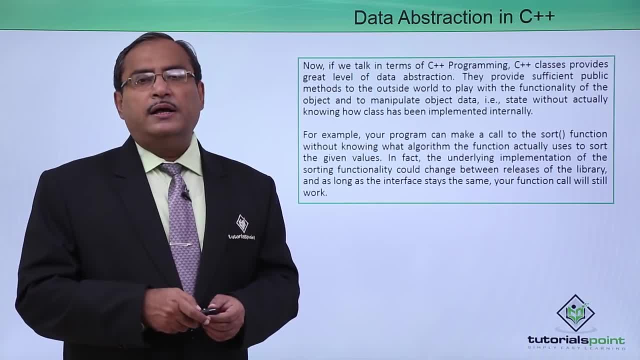 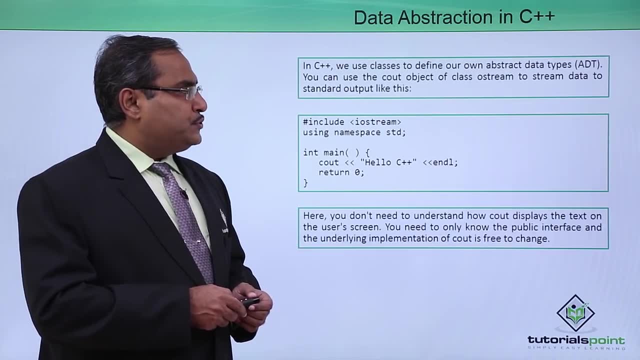 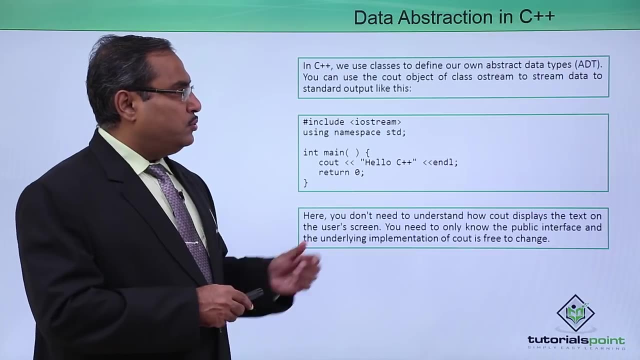 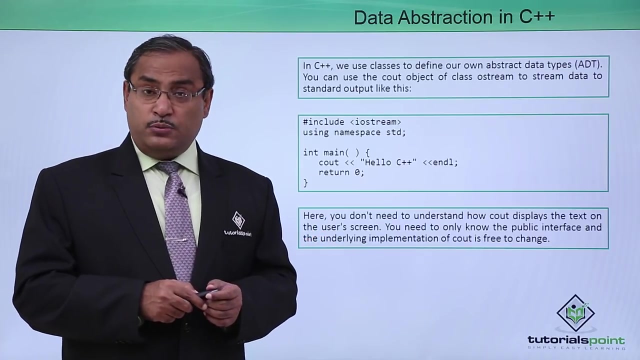 no difficulty to access it without knowing into the algorithm details of the short function in c plus plus, we use classes to define our own abstract data type, that is adt. you can use the count object of class o stream to stream data to the standard output like this. so here is one example we are going to have. so here 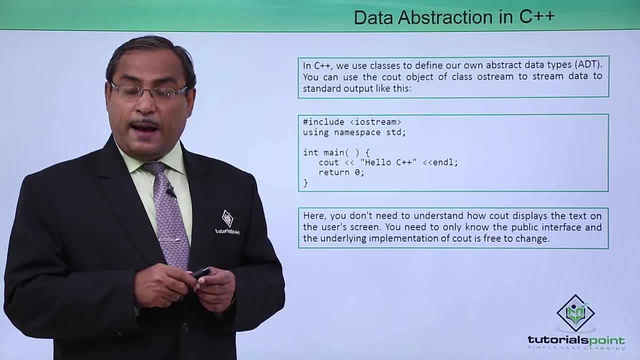 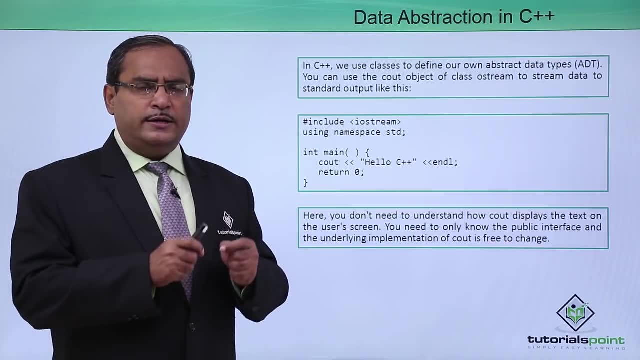 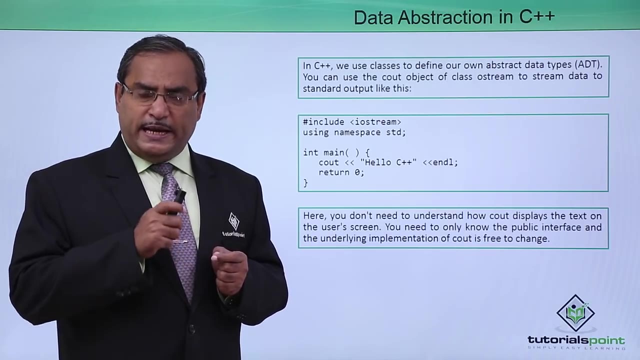 we are giving a birth of another concept, that is, abstract data type. in short, it will be called, as we know that, whenever we define one variable under a data type. so let us suppose we have considered one variable that is int i. so i is a variable of the data type integer. so now we know. 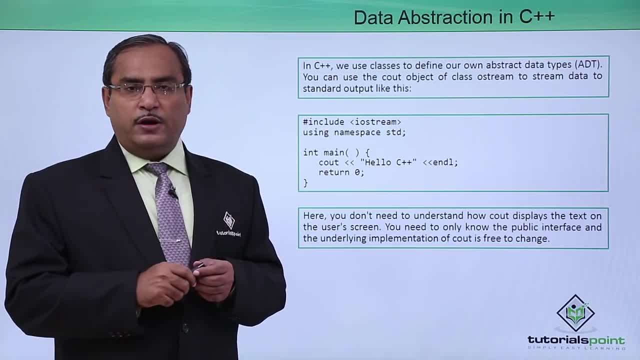 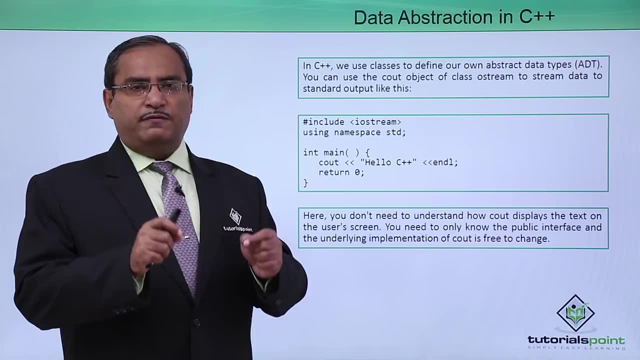 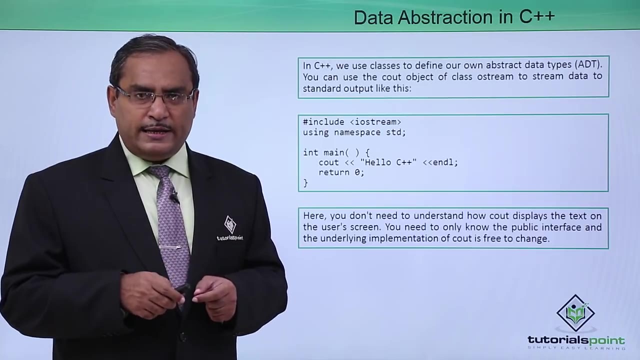 that this i can hold value 10, this i can hold value 20, this i can hold value 100. but if i want to keep one string, say india, onto the variable i, it cannot contain this one. if i keep one value, say 12.45, onto the variable i, it cannot contain that one. so you know that whenever we are having 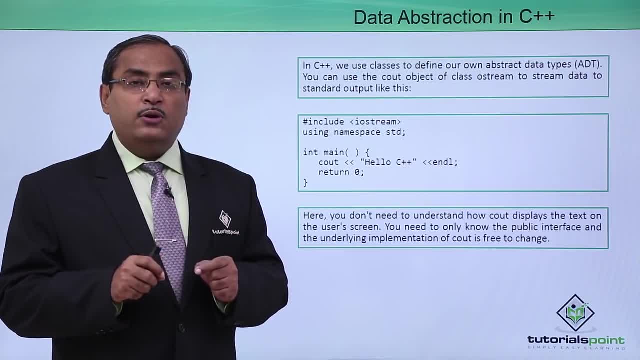 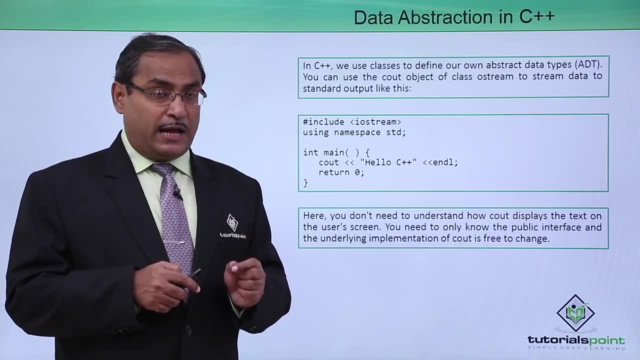 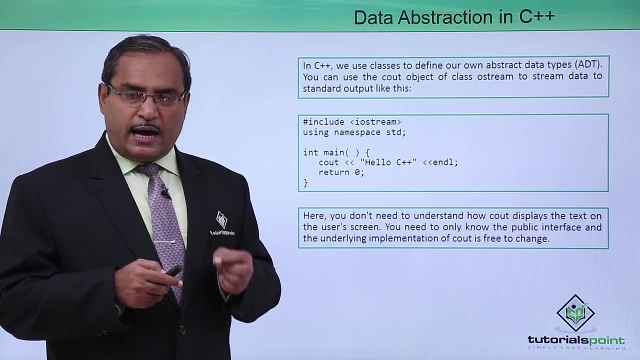 one variable of the data type integer, what value it can hold and what value it cannot hold. let us suppose i want to do addition with this plus with this i, using the operator plus. that can be done. let us suppose i want to do subtraction with this i, that can be done. but if i want to go for lowercase to operand. 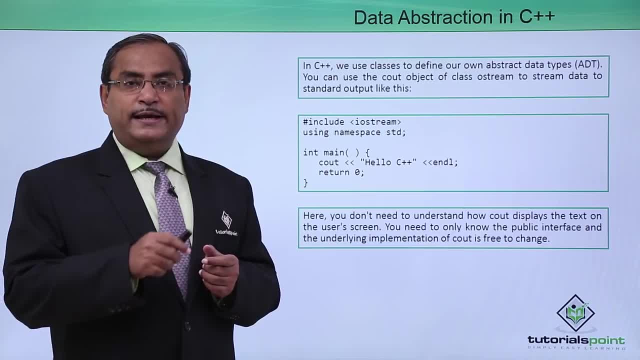 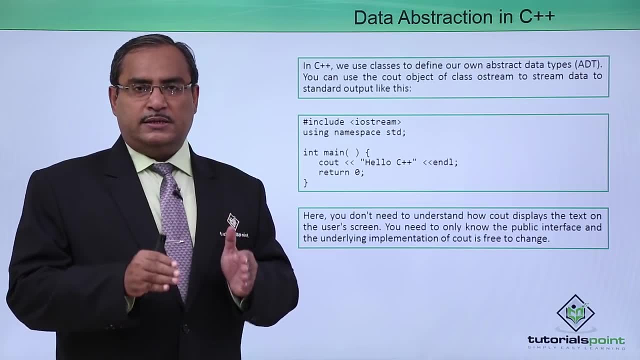 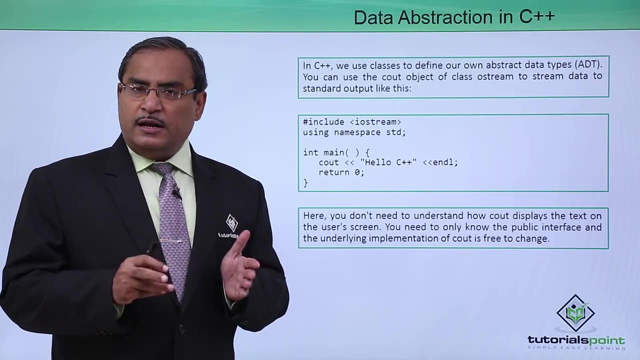 case, conversion from the data which is residing in the variable i. that cannot be done. so also, we know that whenever you are defining one variable i under the data type integer, what are the permitted operations that we can carry out on the variable i? similarly, in case of a class, a class will be. 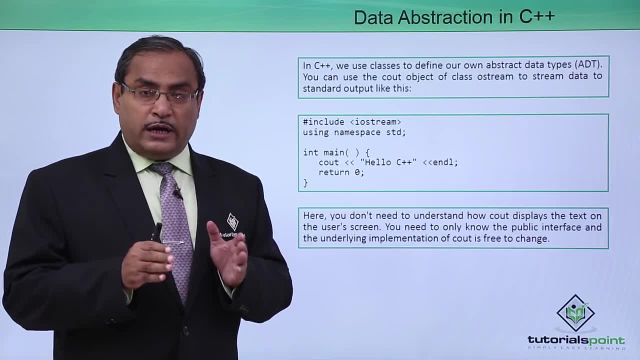 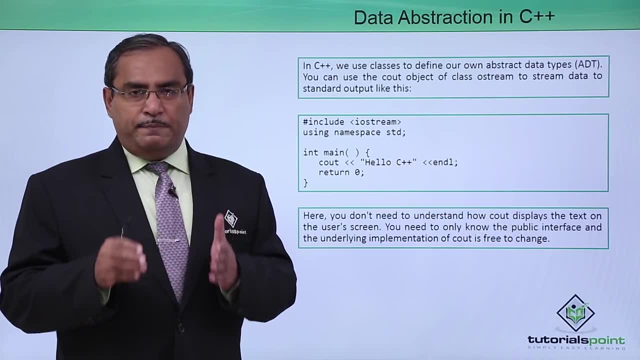 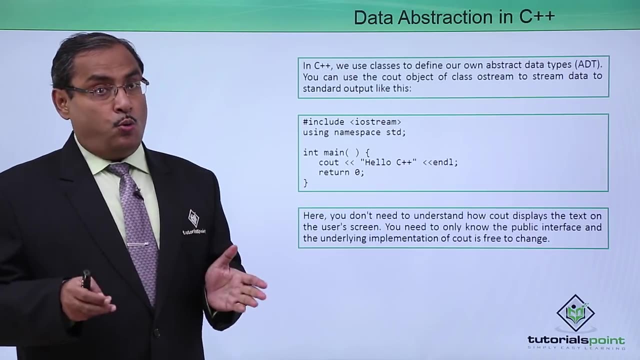 containing different member variables. so we know that, what are the values it can hold and what are the operations we can carry out on them. that will be depicted in the member methods. so, depending upon the algorithm written in those member methods, what are the operations we can carry out with that? 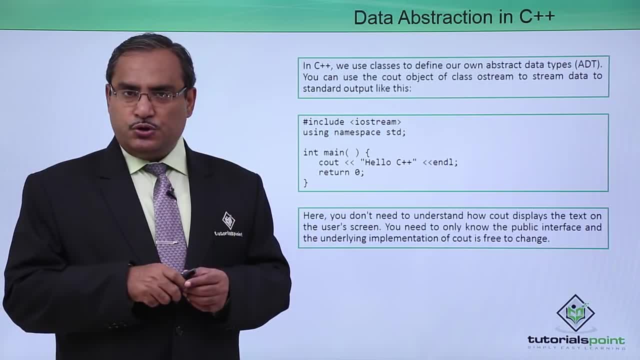 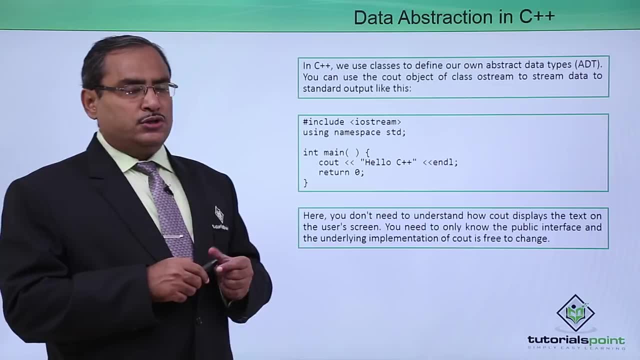 particular class member variables. that is also known to us. so that's why we are going to give a birth of new concept that is abstract data type. so let us discuss this program at first. so here you are, having this cout which is printing this respective structure, and we are going to give a new concept that is abstract data type. so let us discuss this. 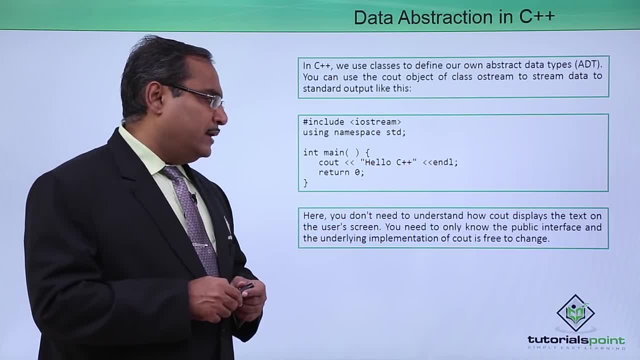 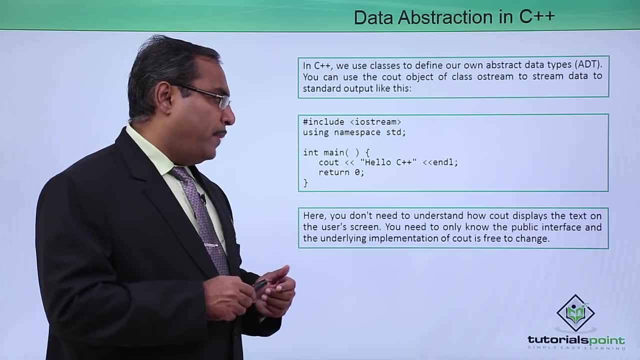 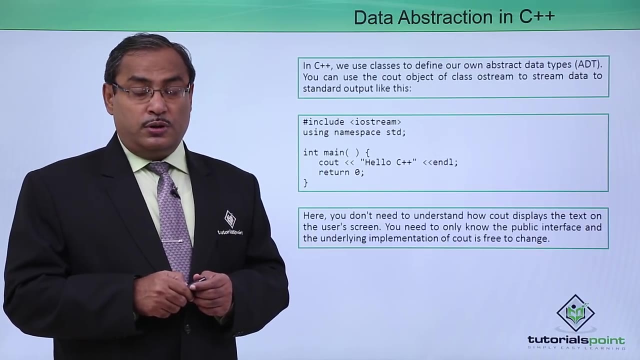 string and so on. here you do not need to understand how cout displays the text on the user screen, you need to only know the public interface and the underlying implementation of cout is free to change, so it the different values of the library functions the function bodies may get.